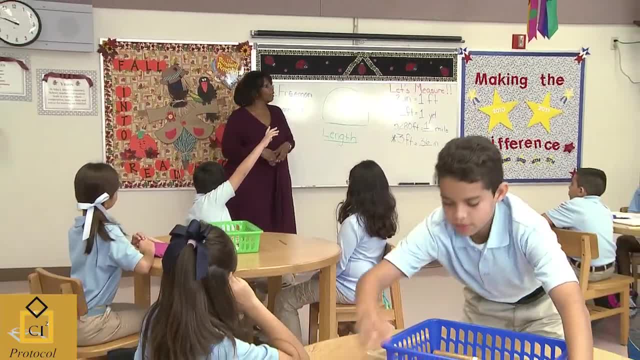 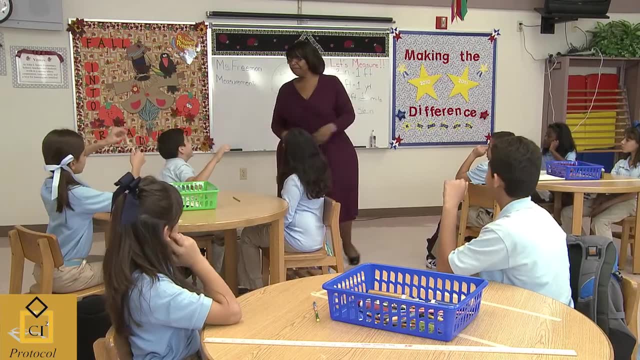 If this did not exist, we didn't have a ruler. We don't have a yardstick. The ruler and yardstick monster came and took them all away. We don't have any more. He came for Halloween. He took them all- Gone. 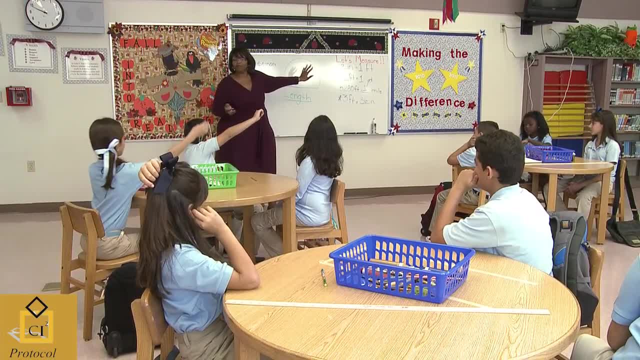 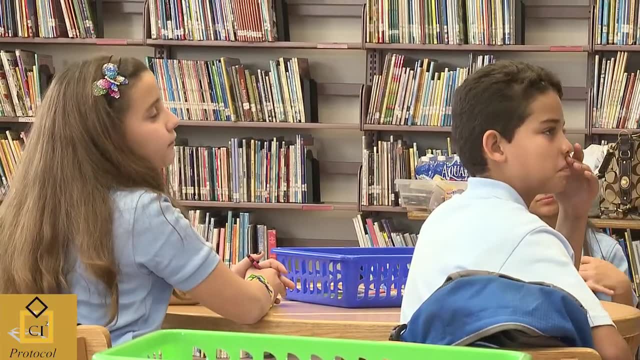 Now I'm still stuck with my problem. I still don't know what to do. I still haven't figured out which one is longer. Alright, What I want you to do, discuss it. Figure out. how would you know which one of these is longer. 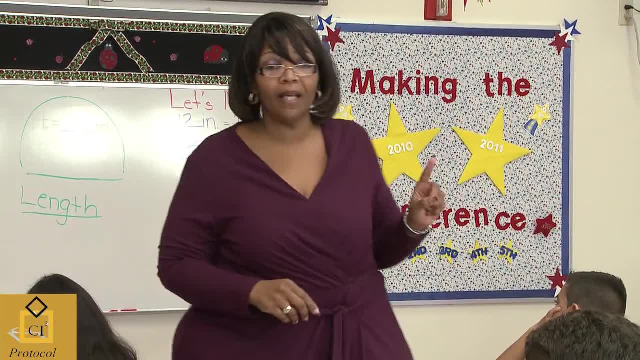 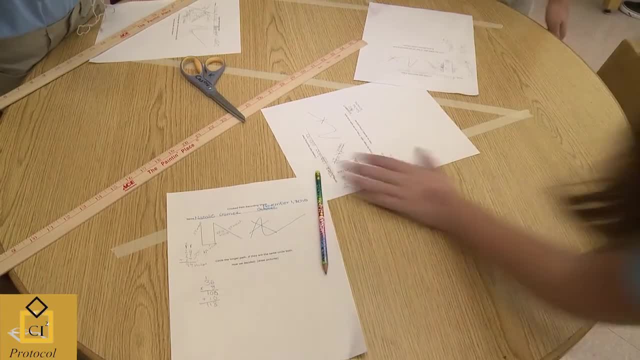 And then one person is going to report to me. One person is going to let me know what your team thinks. Okay, The best strategy or the best way to figure out which one of these lines is the longest. Do we understand the instruction? Yes, 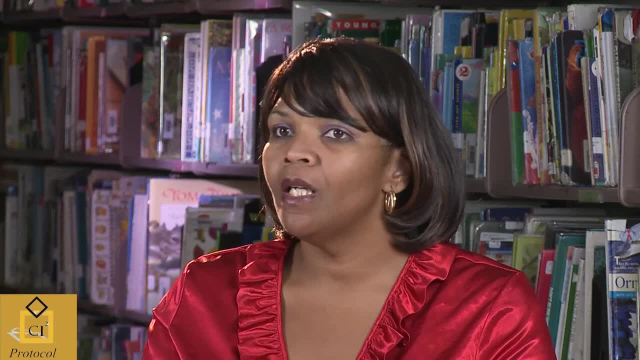 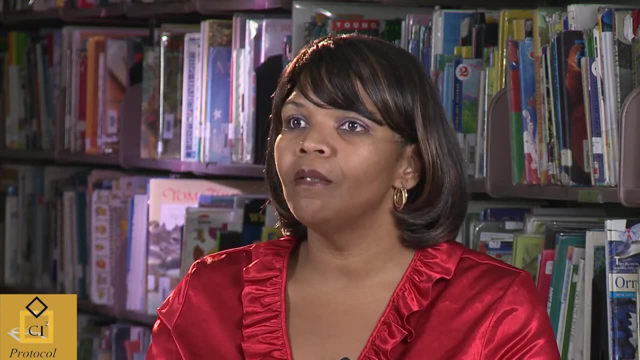 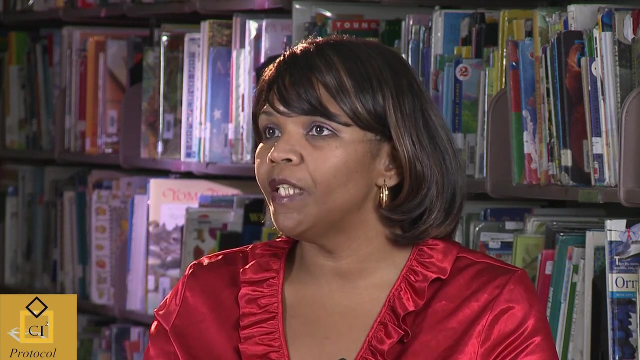 The students need to take ownership and figure it out for themselves. They used the tools that they felt were the best for the activity. They were given pencils, string, yardsticks. All those things were made available to them. However, there was no right or wrong tool to use, So I left it up to them in order to figure it out. 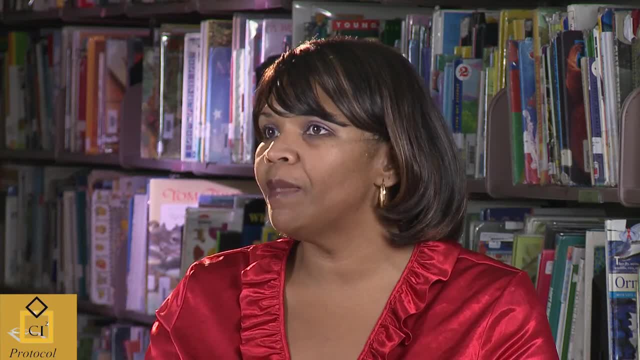 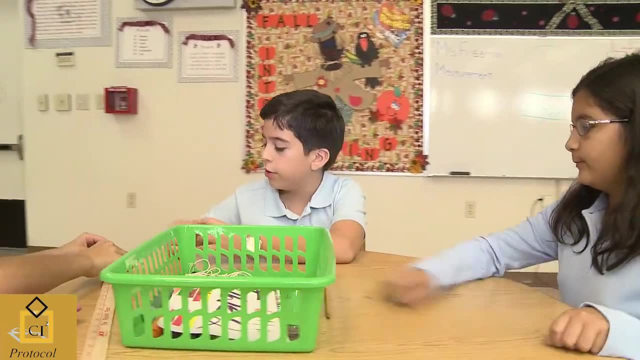 And once they figured out which tool worked best for them, then I just supported them in that decision And allowed them to make their own decisions. We can just use the string and measure it, or put the tip of your nail to your first quarter of your knuckle. 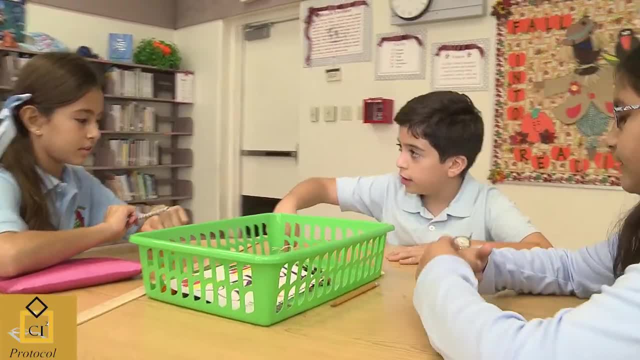 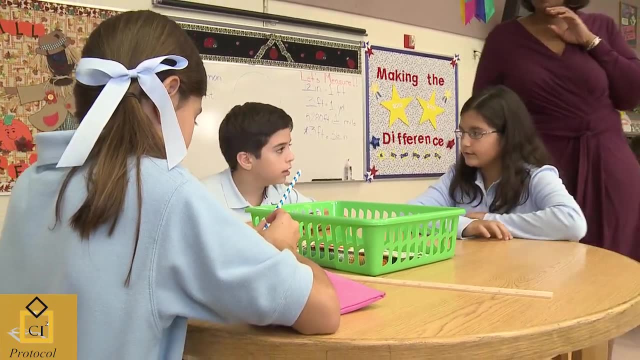 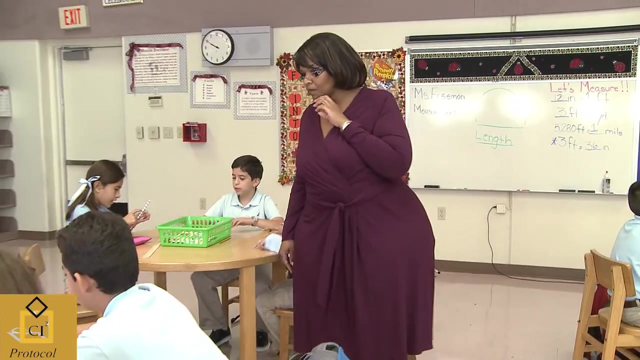 That's an inch. We can measure it like that Or we can just measure it with the other end. So it would be one, two, three. Imagine this is the bottom line right there, And then if we use the string, then if we were straightening it out, the top one would be longer. 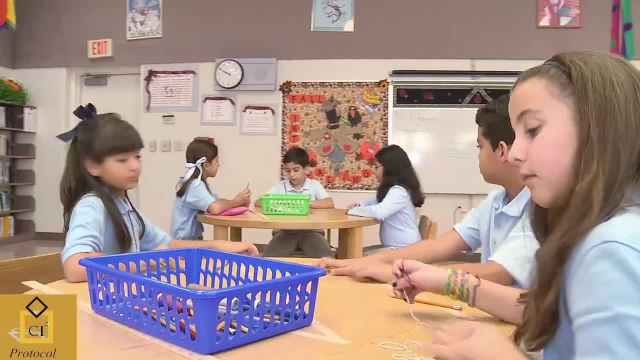 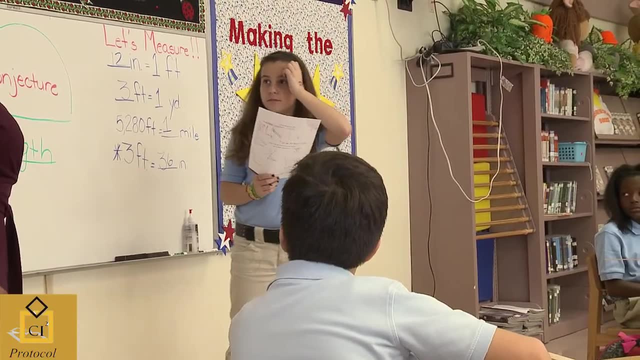 Then we would use the string. So they estimated the size of the first figure And it was going to be larger than that. Okay, so your projection was what? That when I saw the first figure, I saw it and I saw the sizes.